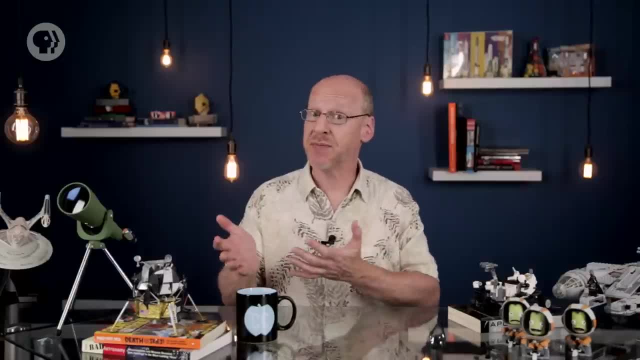 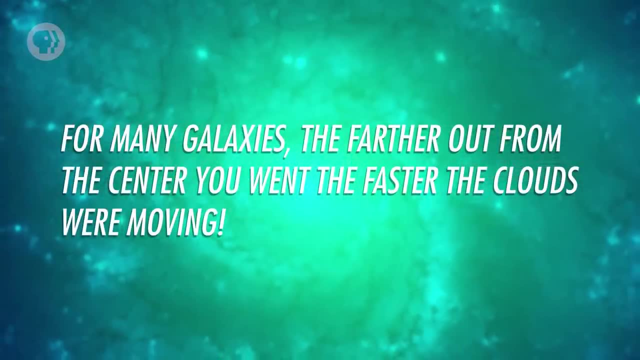 cloud was, the slower it would be moving, just like more distant planets from the Sun move more slowly in their orbits. What she got, though, was the opposite. For many galaxies, the farther out from the center you went, the faster the clouds were moving, Even at 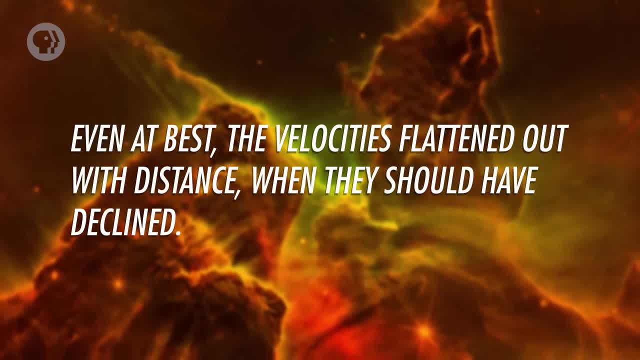 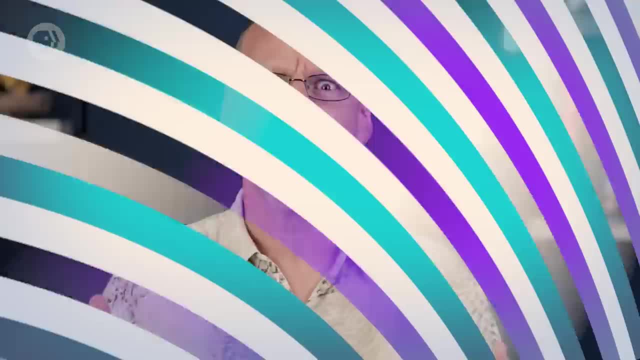 best. the velocities flattened out with distance when they should have declined. That meant the gravity of the galaxies was constant throughout the disk, not dropping from the center as you'd expect, But that's bizarre. Images of the galaxies showed that the number of stars and other massive objects clearly got lower the farther. 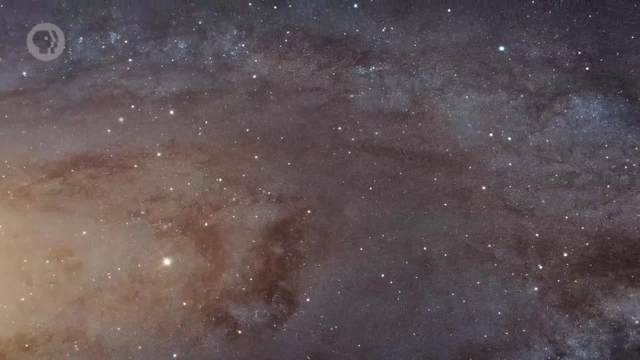 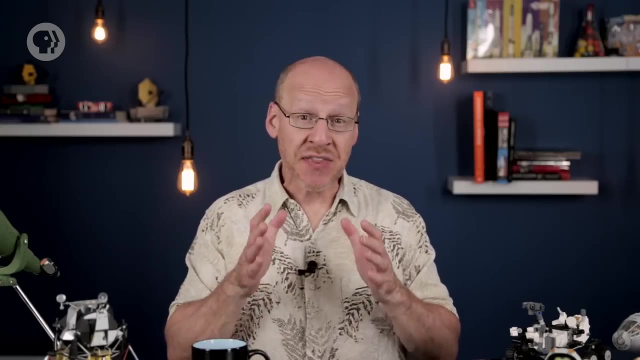 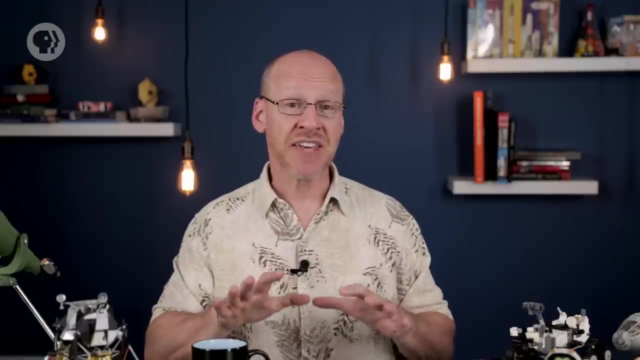 from the center you went. There simply isn't enough mass far out from the center to account for the rapid rotation rates, Or not enough mass from things we can see. The only explanation is that there must be dark material contributing to the gravity — something besides stars, gas and dust. Not only that, the galaxy must be embedded. 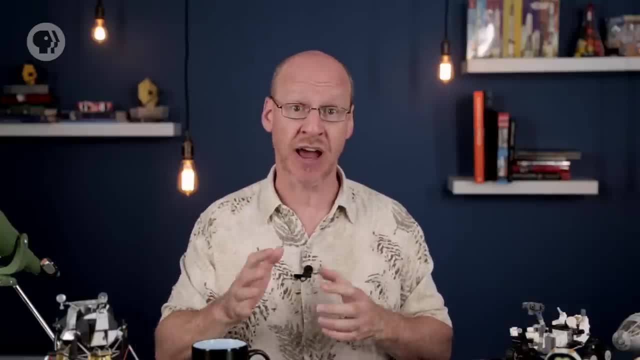 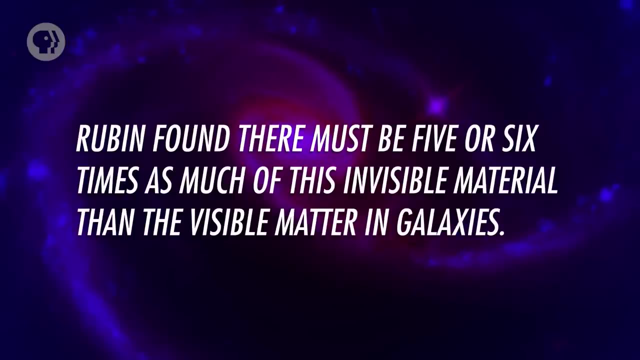 in a halo of this material to get the shapes of the rotation graphs right. And there must be a lot of it. Rubin found that there must be five or six times as much of this invisible material than the visible matter in galaxies. Back in the 1930s, astronomer Fritz Zwicky 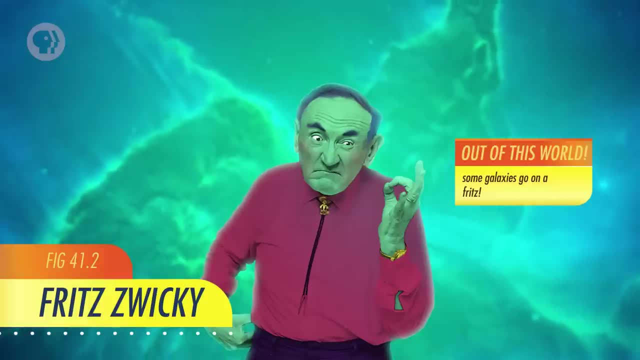 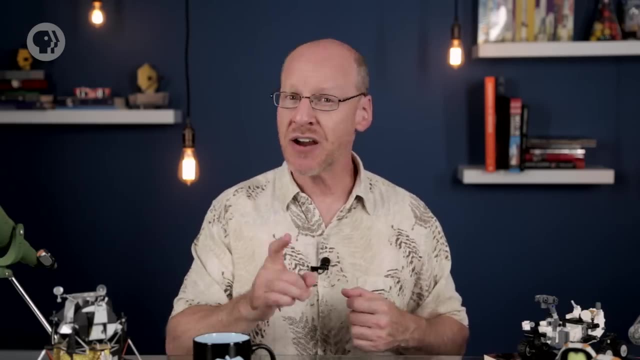 had drawn a similar conclusion. measuring the speeds of galaxies in galaxy clusters, The member galaxies were moving too quickly to stay in the cluster. At the measured speeds they should have been flung off. Therefore, he concluded there must be far more gravity in the clusters than just from. 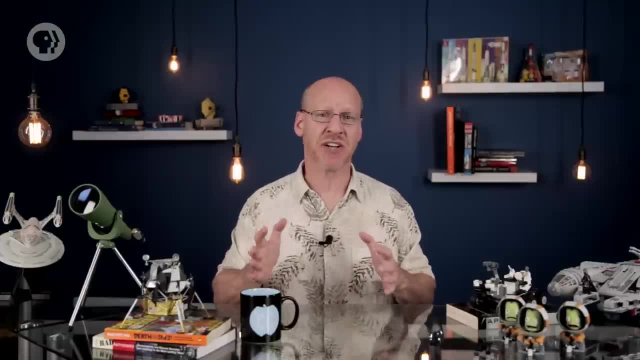 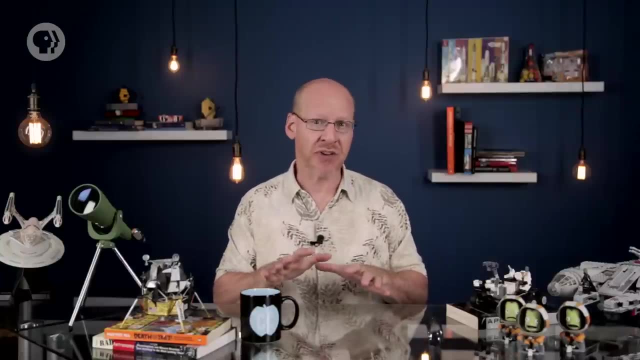 the visible material. It turns out Zwicky's observations had way too much uncertainty in them to make any solid claims. He hugely overestimated the amount of invisible material. Rubin's observations were far, far better and more accurate. However, the term Zwicky used to dub this mysterious 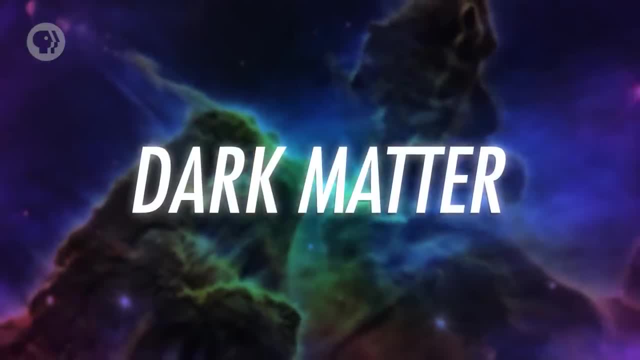 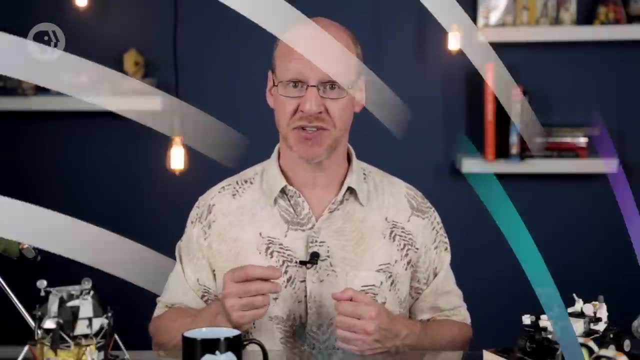 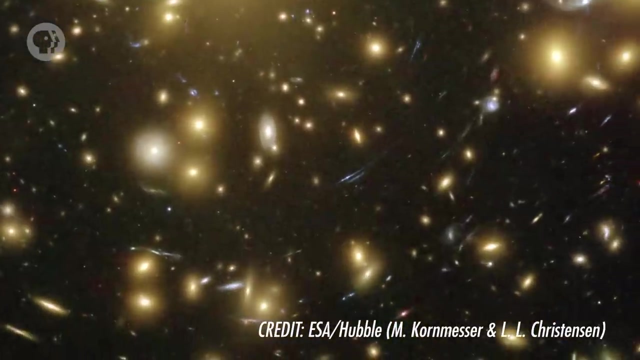 material stuck And we still use it. Dark matter. Over the years, more observations have only confirmed Rubin's measurements. We see similar behavior in elliptical galaxies, for example. Ironically, better measurements made of galaxy cluster member velocities show they do in fact move too quickly And clusters 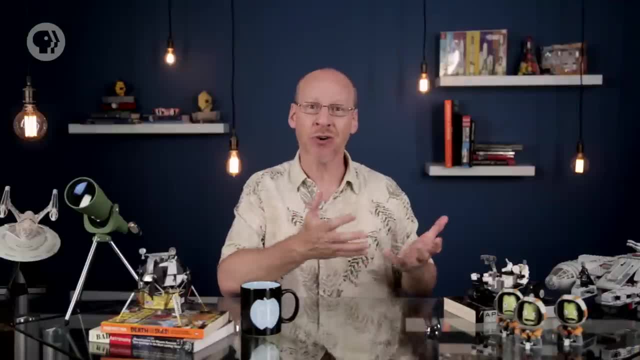 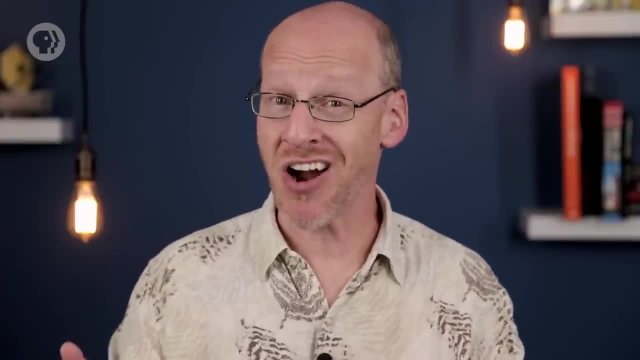 must have dark matter in them too. Zwicky was right for the wrong reason, And in the end Rubin is credited for making the discovery. Of course, the idea that so much of the material in the universe must be dark was met with. 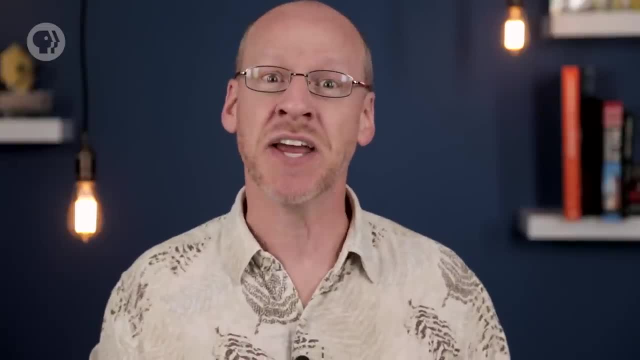 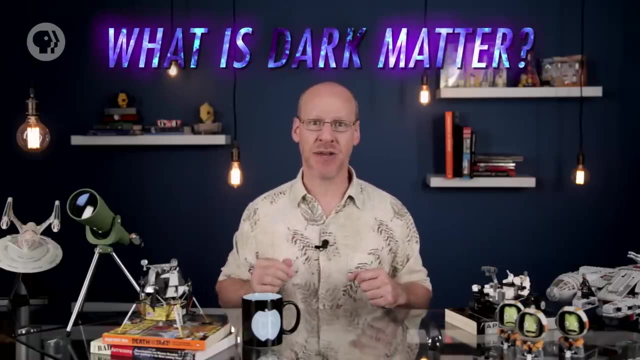 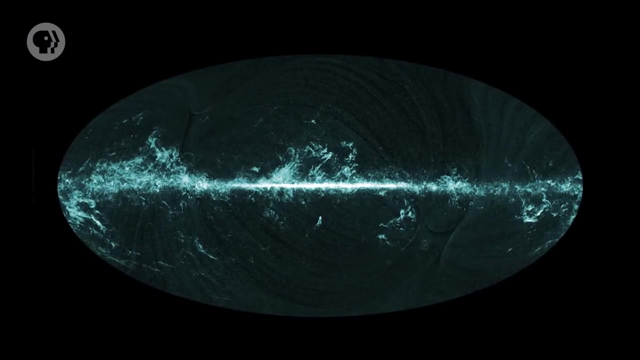 skepticism by astronomers. Everything gives off some kind of light, but more observations just kept supporting the existence of dark matter. So what is dark matter? That was the big question. Astronomers were methodical. They listed every single thing they could think of that dark matter could possibly be Cold gas dust. 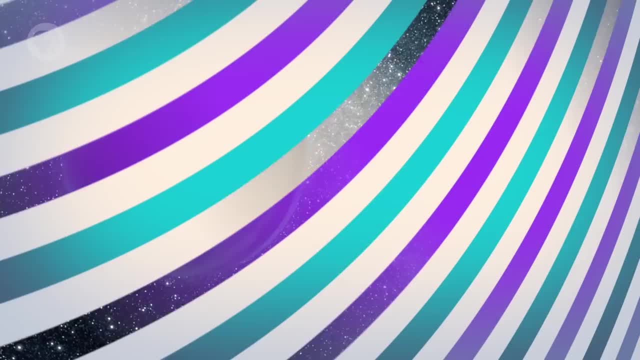 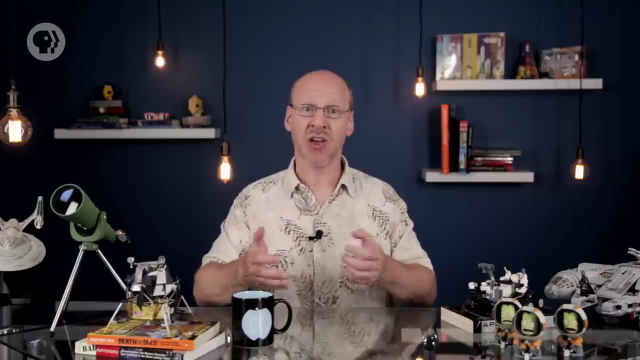 dead stars, rogue planets, everything, Even weird subatomic particles that were predicted to exist in quantum mechanics theories but never seen before. Then they thought of ways they could detect these objects: Cold gas would emit radio waves, for example, But everything. 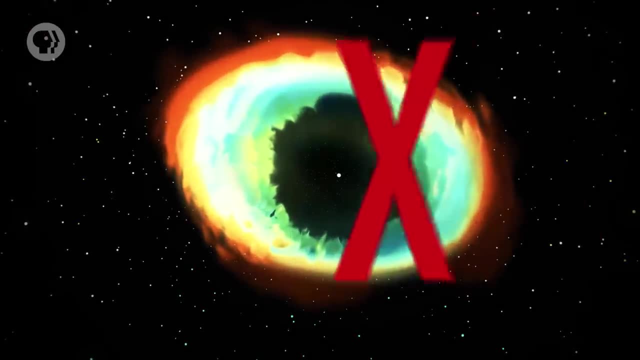 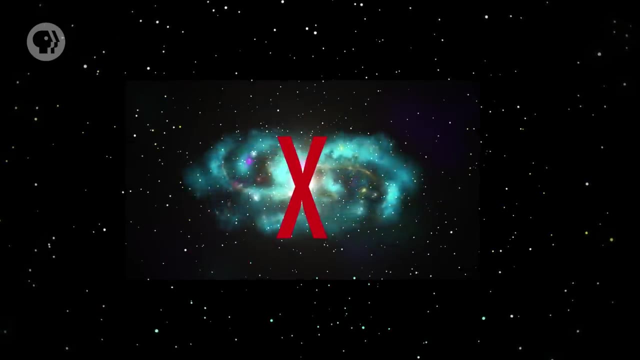 they tried came up empty. One by one, they crossed objects off the list and eventually abnormal matter — atoms and molecules, protons, electrons and neutrons — was eliminated. All that was left on the list was that truly bizarre stuff: those screwy subatomic particles. 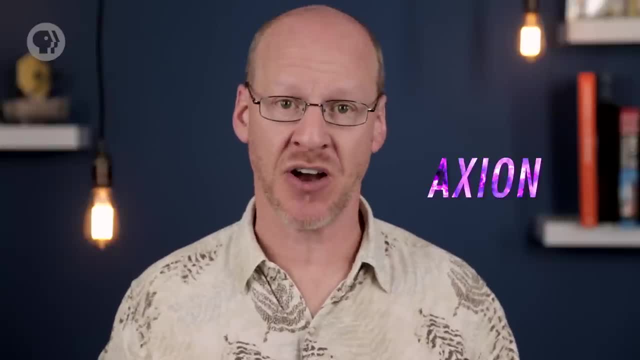 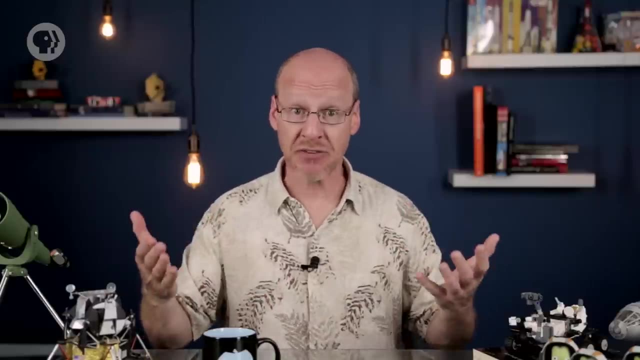 no one had ever seen before. One such particle is called an axion. They've never been detected, but their properties match what we see of dark matter. Axions have mass, so if you have a huge cloud of them they'll have enough gravity to affect galaxies. They don't tend. 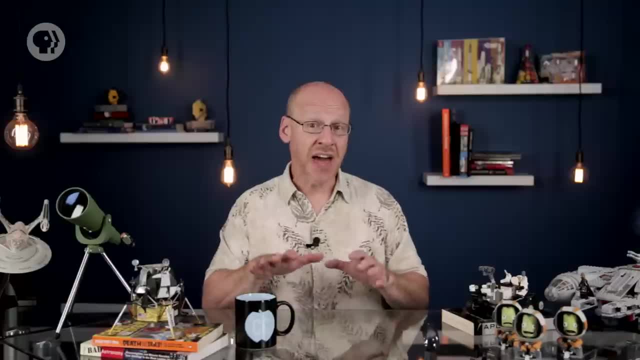 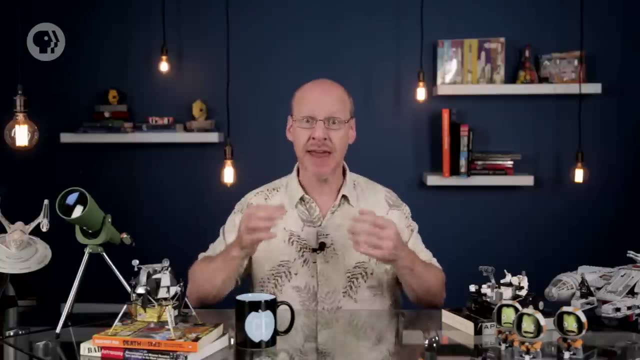 to emit much light, so even a huge cloud of them would be dark. And they have another weird property: They don't interact with normal matter terribly well. An axion would pass right through you like you weren't there. If dark matter were made of axions, then clouds of it can be enveloping. 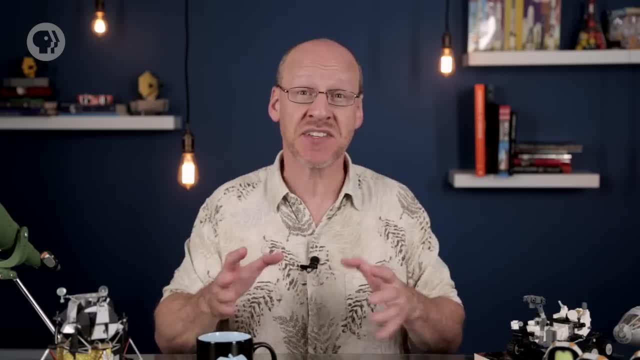 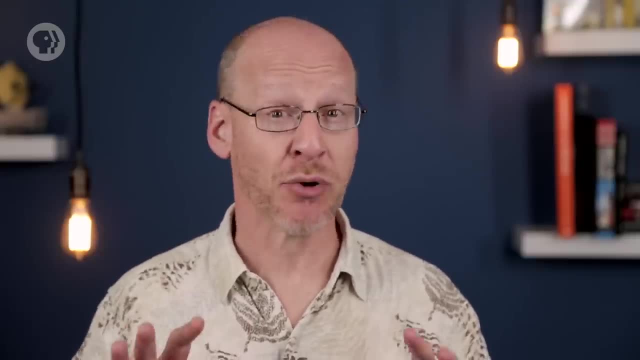 clusters of galaxies and we'd never see them. If that's the case, how could we ever know if they're there or not? It turns out there is a way, But before I talk about that, we have to go over something pretty weird, Actually several somethings weird. 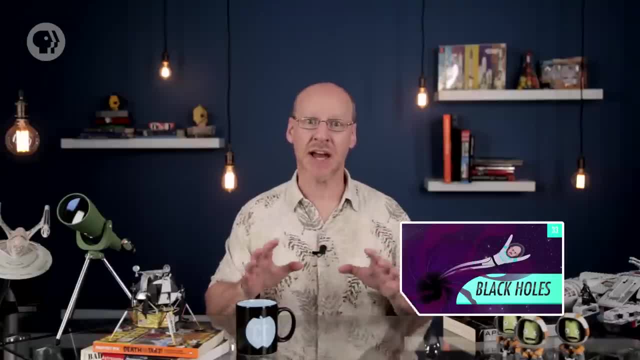 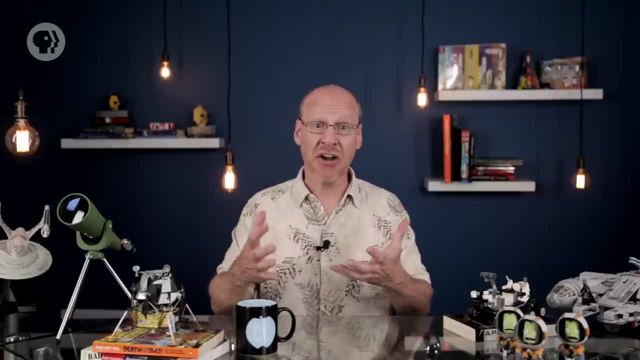 As I mentioned in our black hole episode, one of Albert Einstein's big ideas was that space wasn't just emptiness between stars. It was space. Space wasn't just emptiness between stars. In a sense it was an actual thing with all of matter and energy embedded. 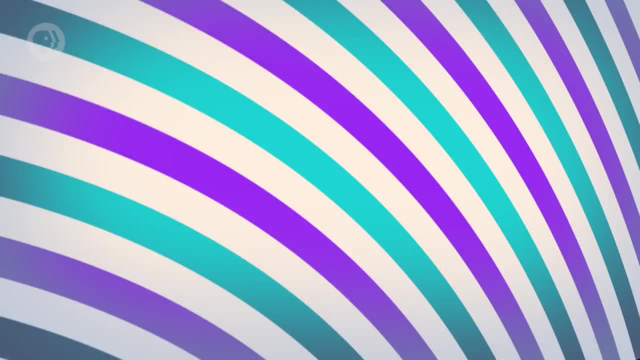 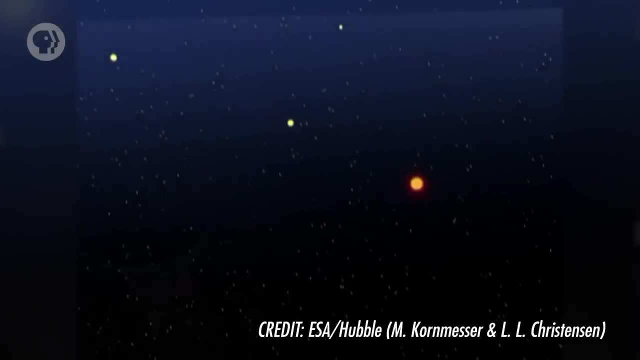 in it, Although you have to be careful not to take the analogy too literally. in many ways, it acts like a fabric with everything stuck to it. This is more than just a theoretical construct. It has real implications For one, what we perceive as gravity, the force pulling two. 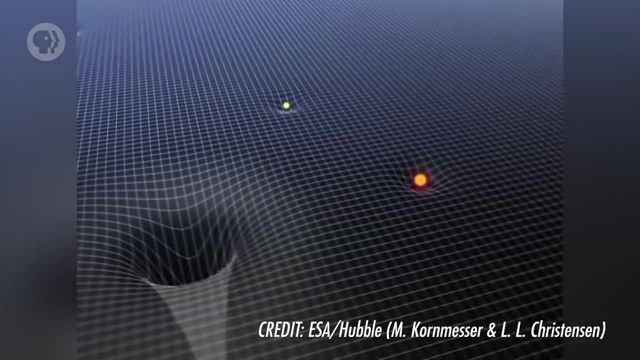 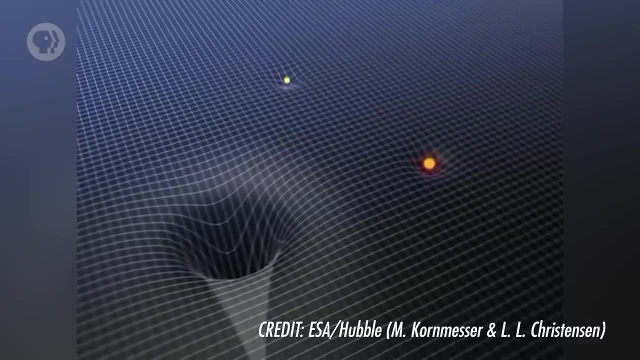 objects together was actually just a bending of this fabric of space, a warp. It's like a bowling ball sitting on a soft mattress. The surface of the mattress bends and if you roll a marble past it, the path of the marble will curve. This is true for light too. It's like having a bend in the road. Cars follow the bend as they move, and trucks do too. Everything does With light it doesn't bend nearly as much as matter does, but it does curve if it moves through space distorted by gravity. 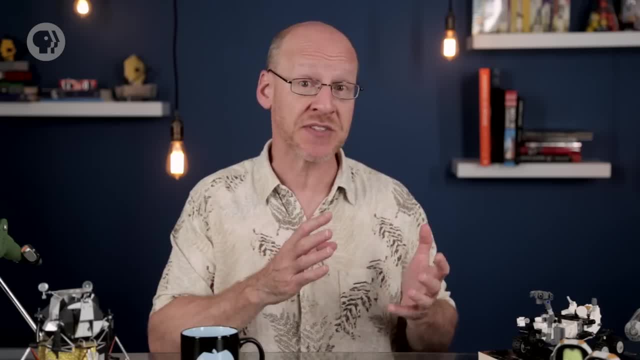 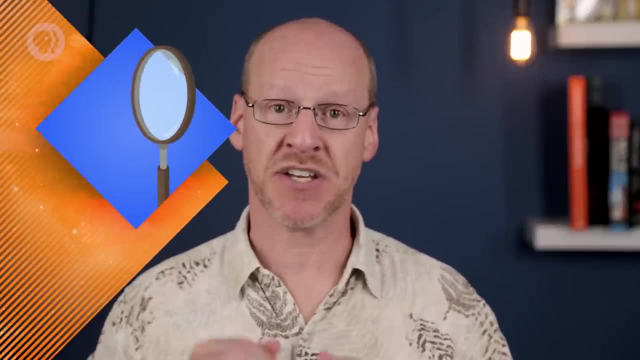 The more massive an object is, the more gravity it has, the more it warps space and the more it can warp the path of a light beam. You know what else bends light? A lens. So we call this effect gravitational lensing. 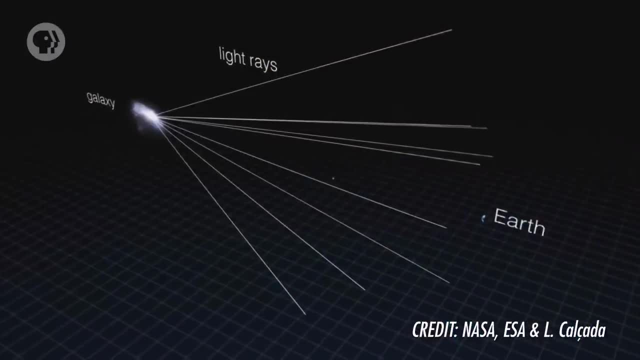 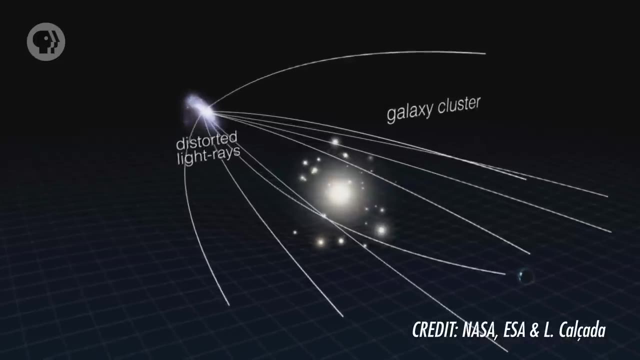 Now picture a cluster of galaxies. It has a lot of mass and a relatively small amount. Well, in cosmic terms, If there's a galaxy on the other side of the cluster, from us, much farther away, the light that more distant galaxy sends out gets bent on its way to us. 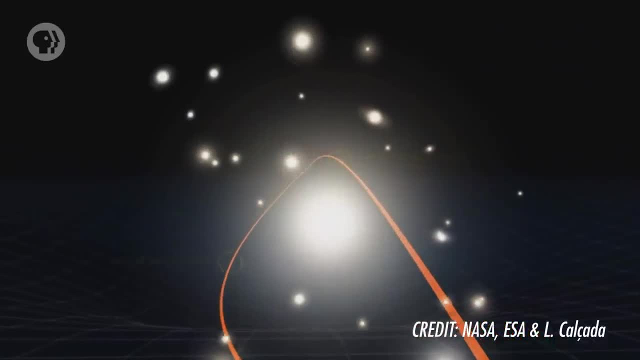 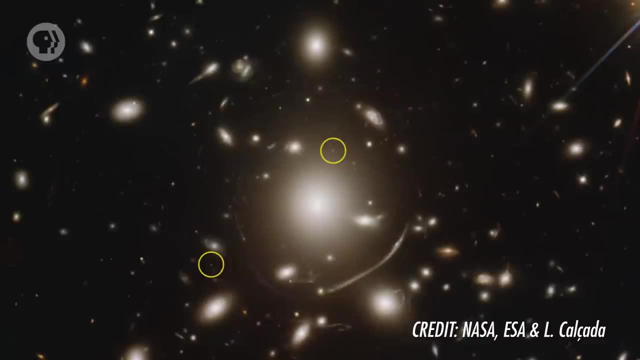 The image of the galaxy can get smeared out, distorted, forming fantastic and weird shapes. Einstein's equations tell us that the amount of bending depends on the mass of the cluster. So we can in theory measure the mass of the cluster by the distortion of objects behind. 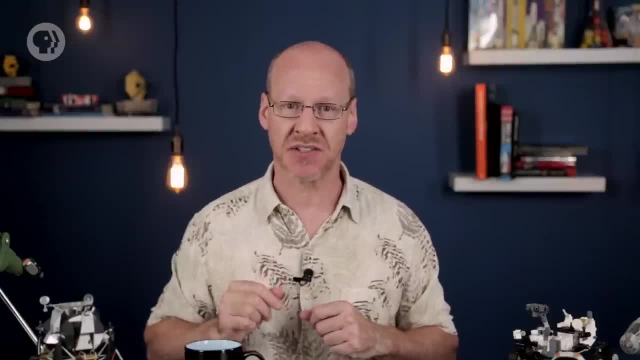 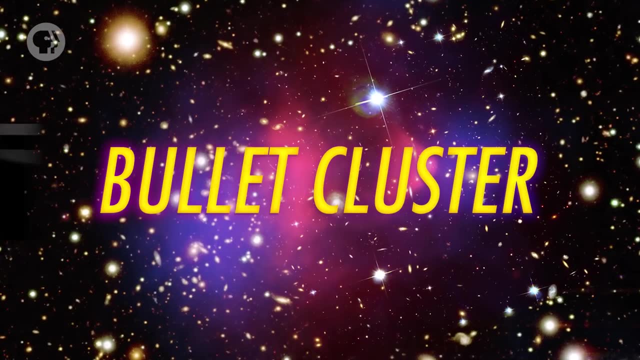 it. Not only that, but it gives us a map of where that mass is. Astronomers use this method on a cluster of galaxies. There's a cluster of galaxies located about 3.5 billion light-years away called the Bullet Cluster. It's a very special object. It's actually not just a cluster, but a collision. of two clusters. That's right. Two huge groups of galaxies are physically colliding and may eventually merge to form one huger cluster. When galaxies collide they tend to pass through each other like ghosts, But in clusters between the galaxies there are vast amounts of gas. When 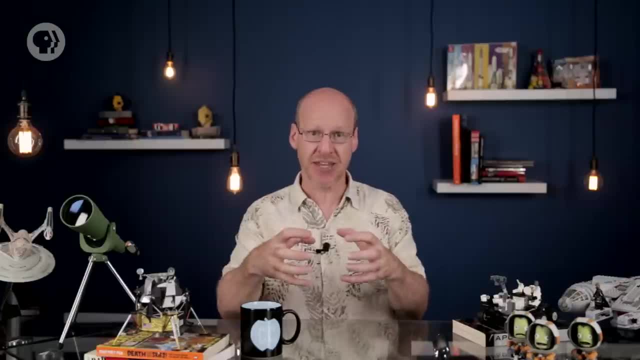 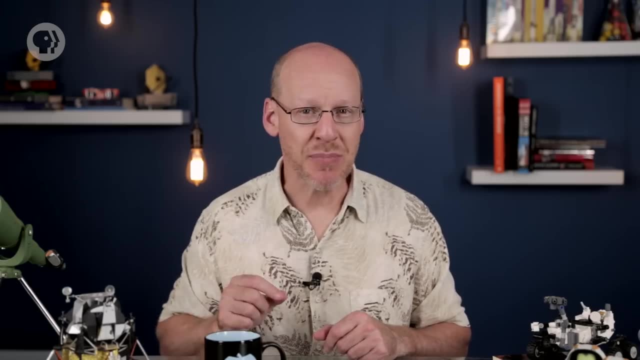 clusters collide. the gas in the two clusters does indeed smack into each other and get incredibly hot, So hot in fact. the gas will emit X-rays. This provides an interesting opportunity. Optical light images show the two clusters next to each other. They've already done one pass, in fact. The galaxies move through. 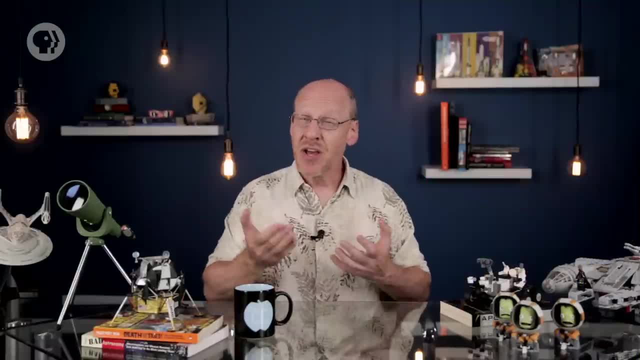 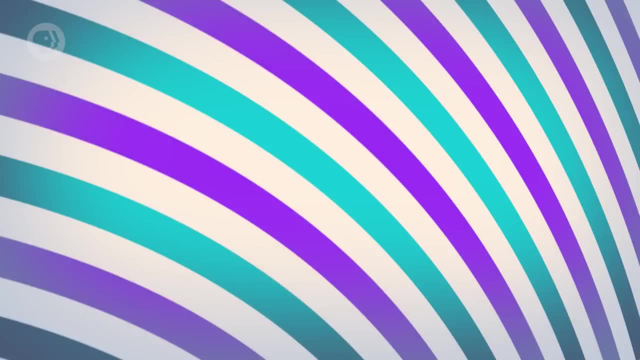 each other. as expected. The gas in the clusters can't do that, though, so you'd expect most of it to be between the galaxies, having slowed down as the clouds collided with each other more or less head on. Using the Chandra X-ray Observatory, astronomers could map out where that hot gas was, And 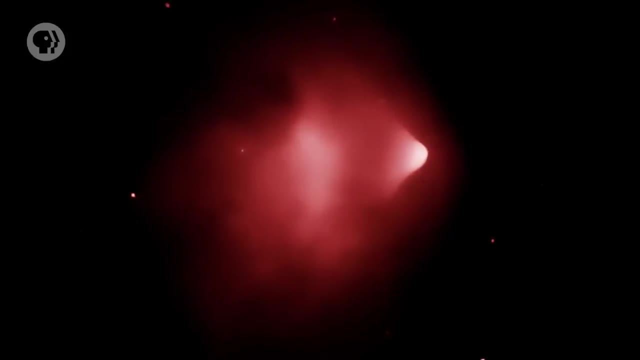 as expected, it lies most of the way between the two clusters. This is a very interesting example of what happens when the two clusters collide, mostly between the galaxies having slowed down after the collision. You can even see how the collision has shaped the gas, forming a bow shock in one cluster. 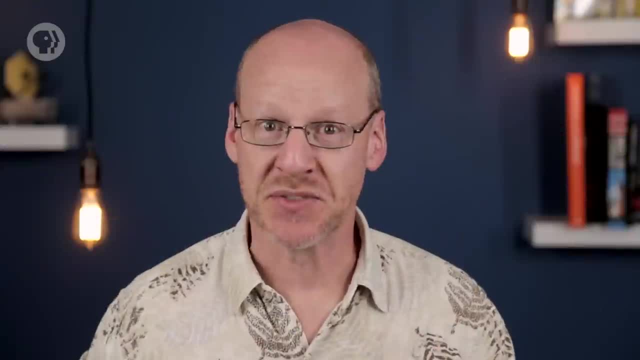 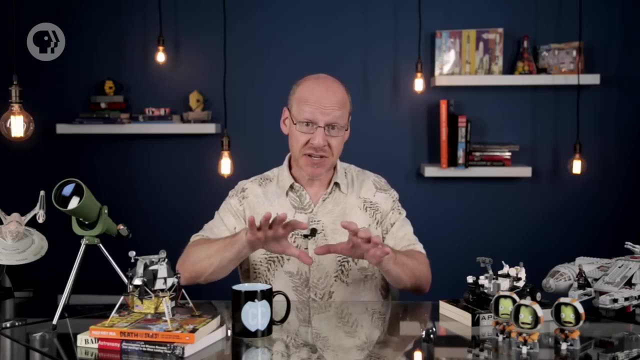 like the waves of water created by a rapidly moving boat. But there's more. Even though the Bullet Cluster is very far away, there are actually hundreds of galaxies even farther away that can be seen in the optical images. The gravity of the matter in the Bullet Cluster distorted those background galaxy images subtly. 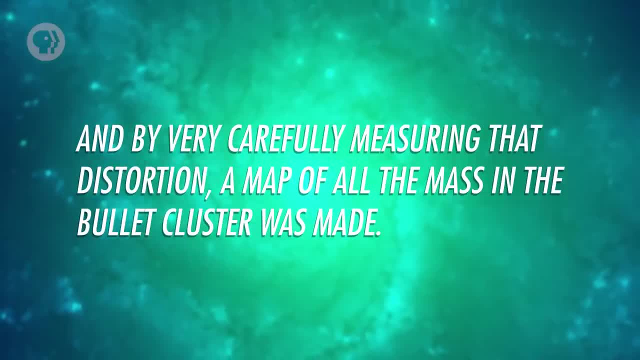 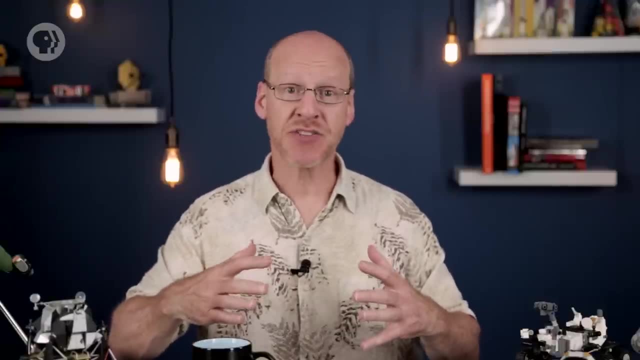 And by very carefully measuring that distortion, a map of all the mass in the Bullet Cluster was made, including dark matter. If dark matter is made of axions, then you'd expect it to mostly be surrounding the sub-clusters themselves because, like the galaxies, the clouds of dark matter, axions would pass right. 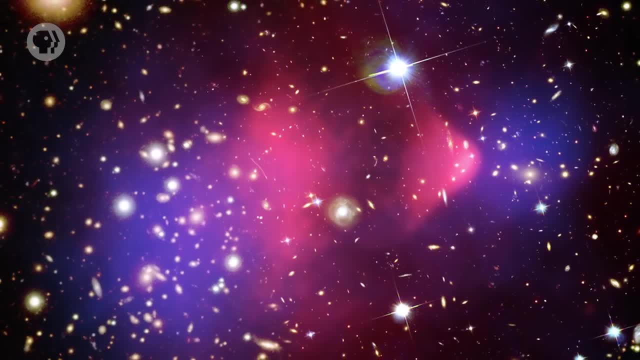 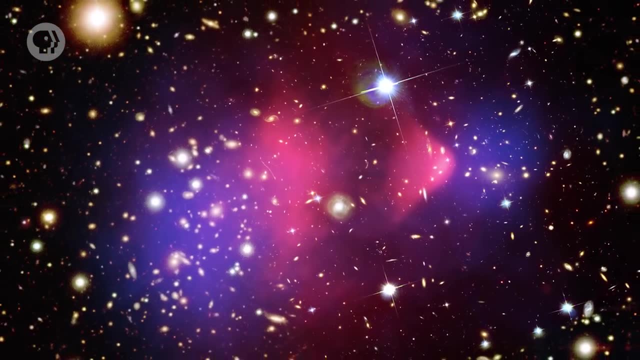 through each other. And when you do make the map, that's exactly what you see. The background galaxies show there's a lot of matter shown here in violet, centered on the two clusters, But it's clearly not the hot gas seen by Chandra and is giving. 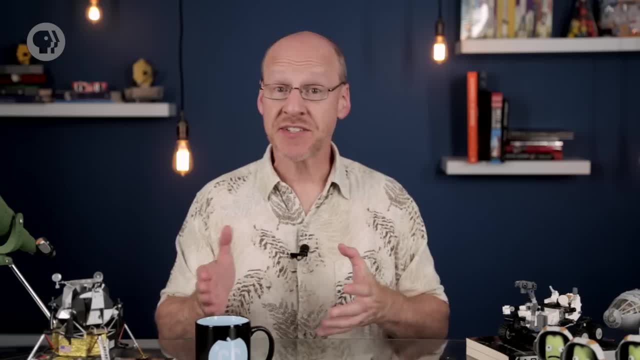 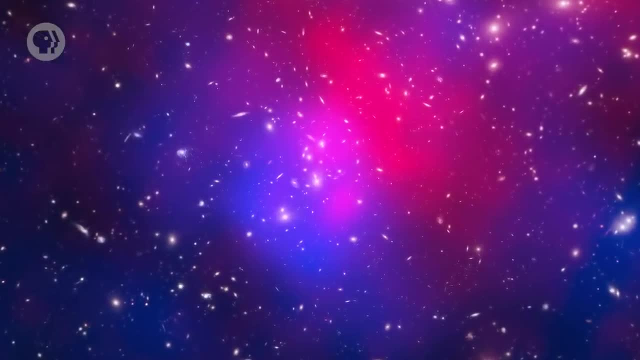 off no light. It looks very much like dark matter. Since the Bullet Cluster observations have been made, we've been able to see that the same sort of behavior has been observed in several other clusters. Attempts have been made to explain these clusters without using dark matter, but in the end 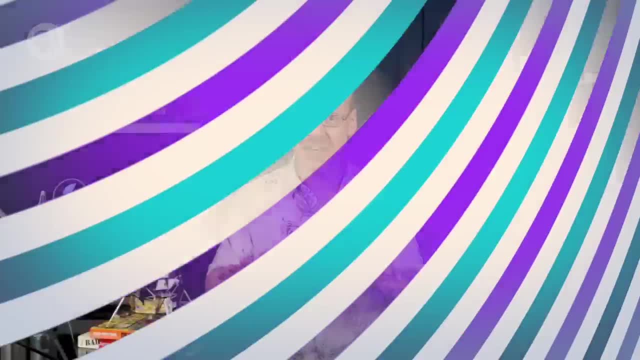 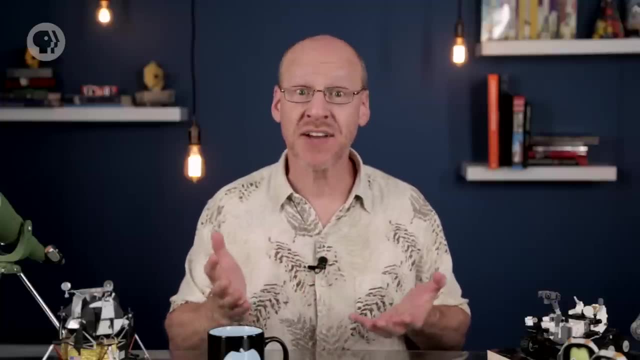 the simplest explanation looks to be the best one. The stuff we see isn't all the stuff there is. To be honest, we still don't know what dark matter is. Axions are one possibility, but others exist. Lots of experiments have been set up to try to detect the various flavors. 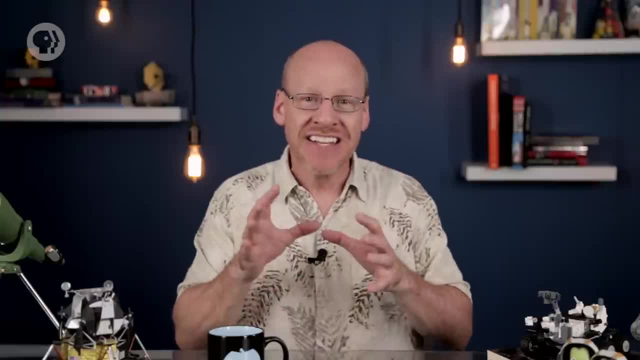 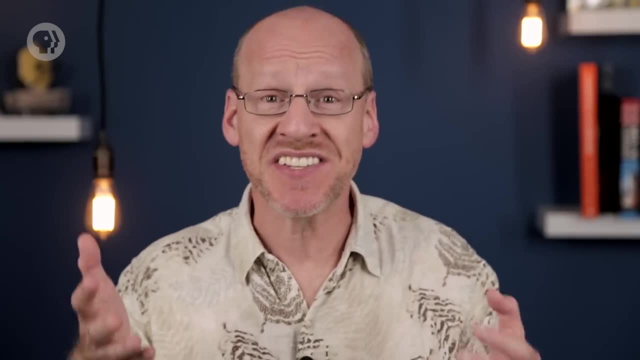 of subatomic particles. but the very nature of dark matter- it doesn't give off light and doesn't interact well with normal matter- makes it really hard to find. That's why it took so long to even know it existed in the first place. 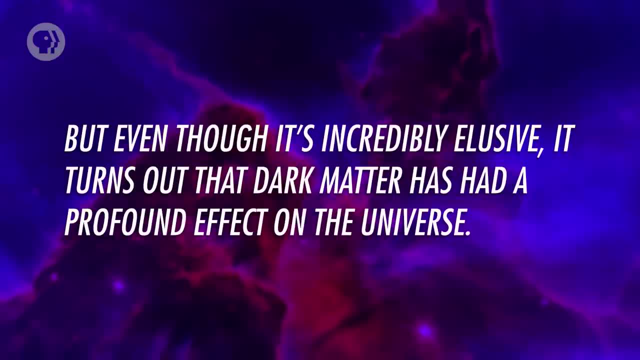 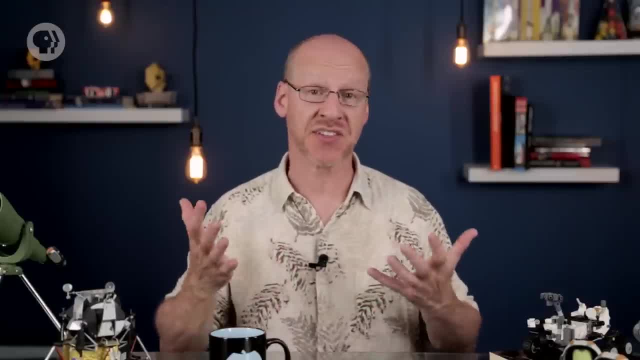 But even though it's incredibly elusive, it turns out that dark matter has had a profound effect on the Universe, As we'll see in upcoming episodes. we're getting a pretty good idea of how the Universe got its start and how it's evolved over the eons, We think 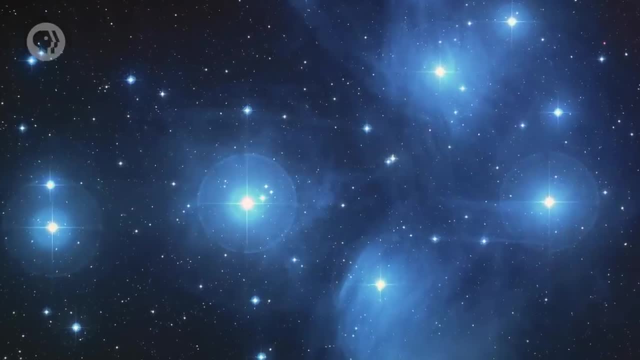 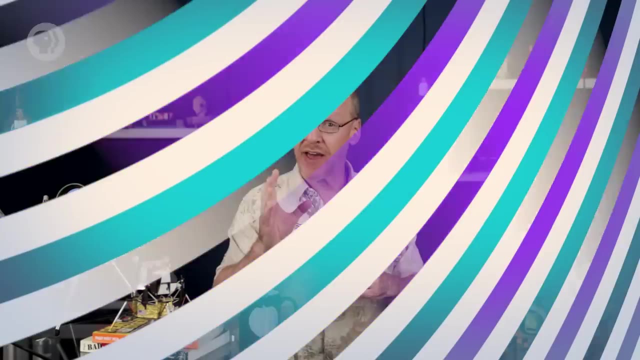 smaller objects formed first, clumping together into larger and larger structures. So stars formed first, then galaxies, then clusters. It turns out that larger structures would have had a hard time forming in the early Universe as energy was blasted out by the newborn stars and galaxies. Bigger stuff couldn't. 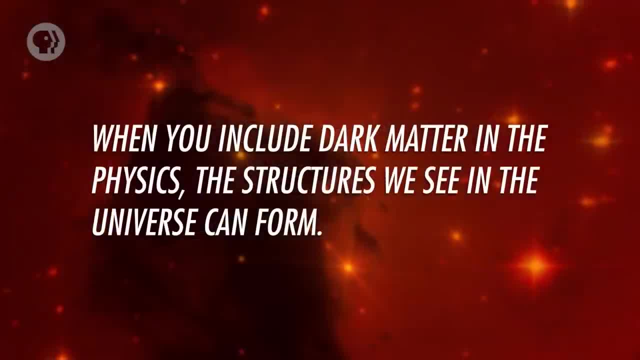 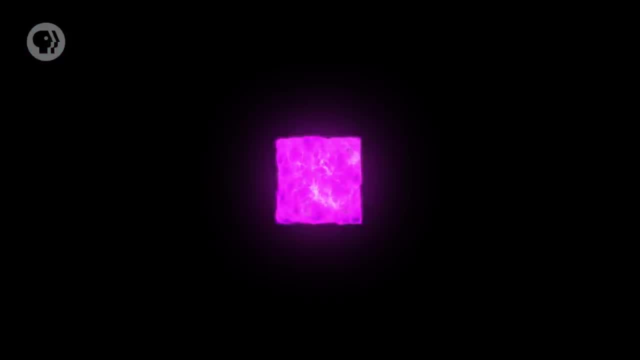 aggregate due to all that heat. That is without dark matter. When you include dark matter in the physics, the structures we see in the Universe can form. How about that? Something like 85% of the matter in the Universe is stuff we can't.